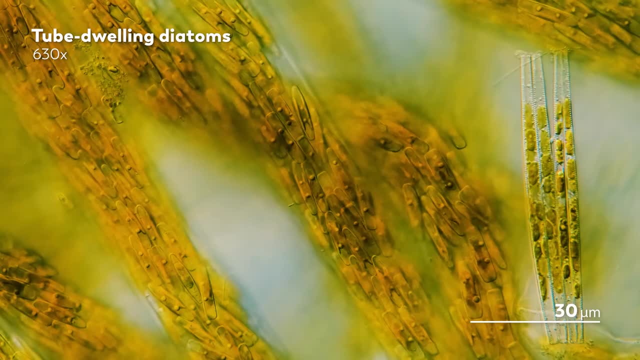 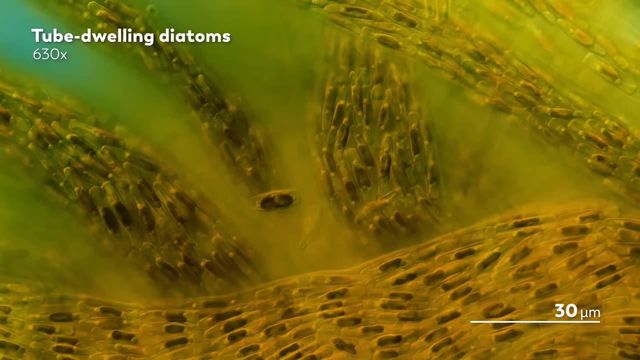 But they saved the marine samples for last, because those organisms tend to be more delicate to handle. So on this last collecting session, James was on a video call watching, as Ella said, and scanned the dock she was standing on And along the submerged parts of the dock James spotted tufts of brownish stuff peeking out as the waves broke. 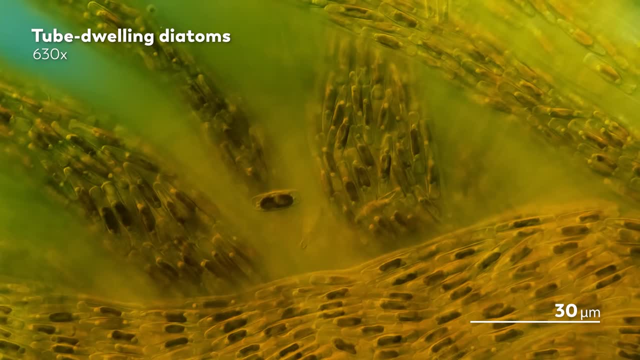 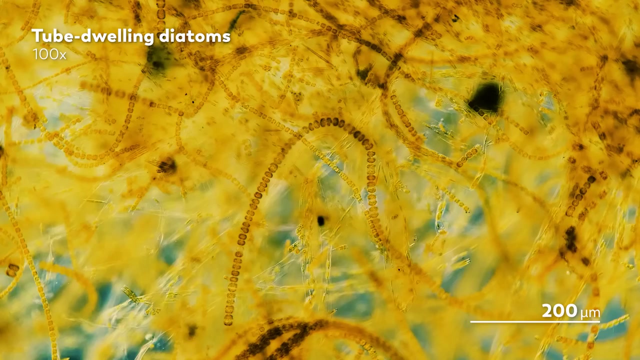 So he asked Ella to grab some and bring them back The next day. she arrived at 6am and crashed on the couch, while James immediately grabbed the samples to take a look, And apparently the entire time he was saying: This is so beautiful. 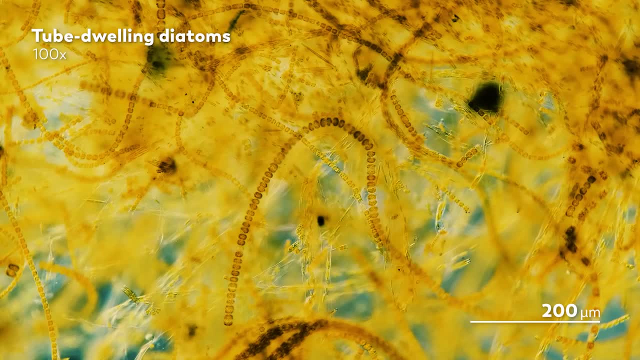 The samples that Ella had found and the samples that James had found were the same samples that Ella had found and the samples that James had found were the same samples that Ella had found. The samples that Ella brought back from the dock were teeming with diatoms. 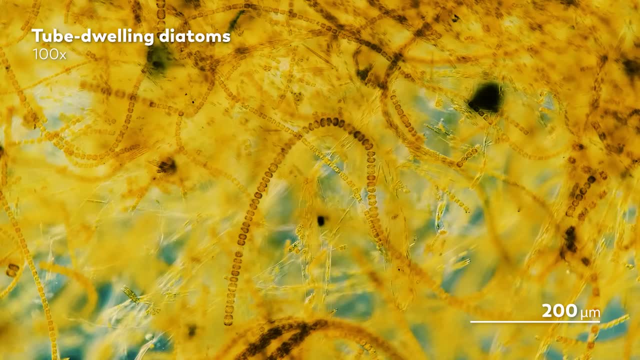 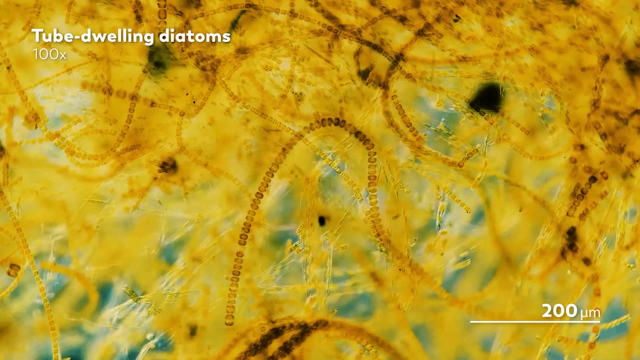 It might seem surprising that the waters of Iceland can bring forth so much life, especially during the cold and dark winter months, But this matches James' experience with the ponds in Poland. he gathers samples from which often end up dominated by diatoms during the winter, even as green algae numbers drop. But this matches James' experience with the ponds in Poland he gathers samples from which often end up dominated by diatoms during the winter, even as green algae numbers drop. But this matches James' experience with the ponds in Poland he gathers samples from which often end up dominated by diatoms during the winter, even as green algae numbers drop. But this matches James' experience with the ponds in Poland he gathers samples from which often end up dominated by diatoms during the winter, even as green algae numbers drop. But this matches James' experience with the ponds in Poland he gathers samples from which often end up dominated by diatoms during the winter, even as green algae numbers drop. But this matches James' experience with the ponds in Poland he gathers samples from which often end up dominated by diatoms during the winter, even as green algae numbers drop. But this matches James' experience with the ponds in Poland he gathers samples from which often end up dominated by diatoms during the winter, even as green algae numbers drop. 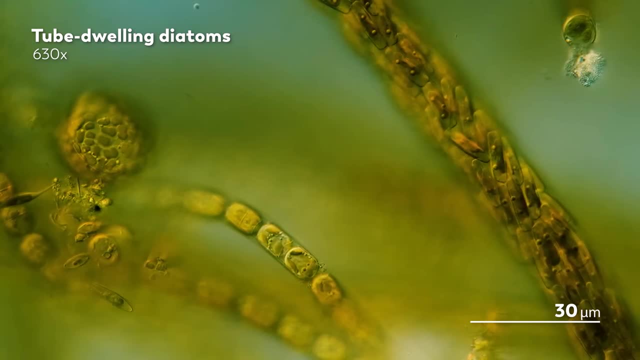 dark. One study found that diatoms survive longer than flagellates in extended periods of darkness. The researchers didn't find a specific reason why they're able to tolerate the dark for so long, but they theorized that perhaps the diatoms were more conservative in how they managed energy. 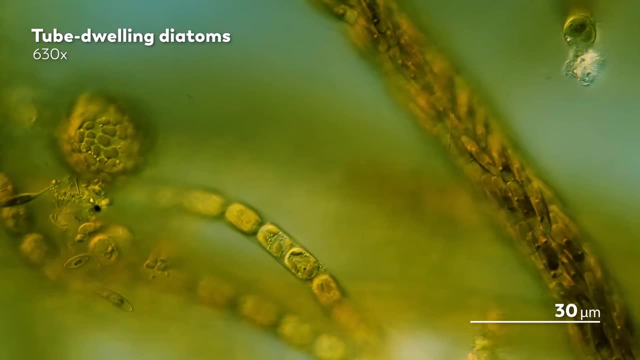 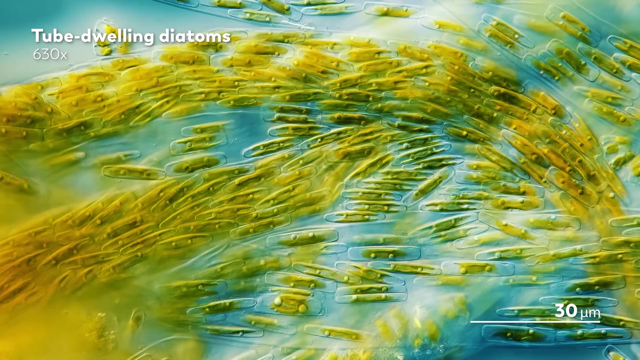 reserves. Others have also suggested that their survival might be due to oil stored in the diatoms, which may keep them better stocked compared to other organisms. Their survival in winter means that when spring rolls around, diatoms are often the first groups to bloom in polar waters. 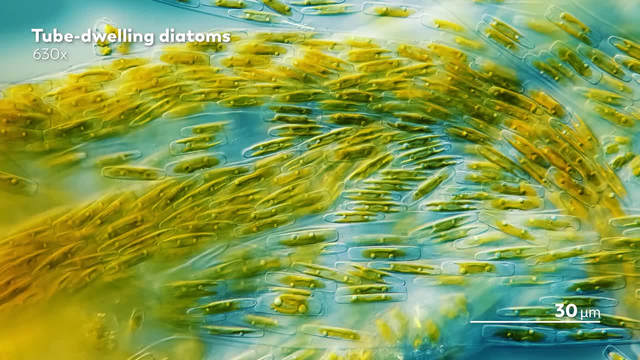 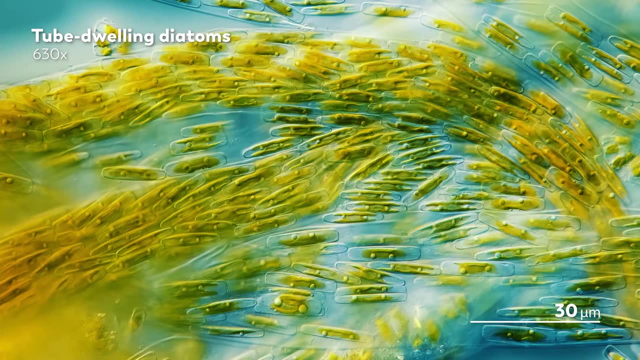 And perhaps these tube-like structures are part of their success. They're not found as often in warmer waters, but things are different when it gets cold. In 1994, a scientist found a whole bunch of these tubes along the Dutch coast in late winter, And by a whole bunch. 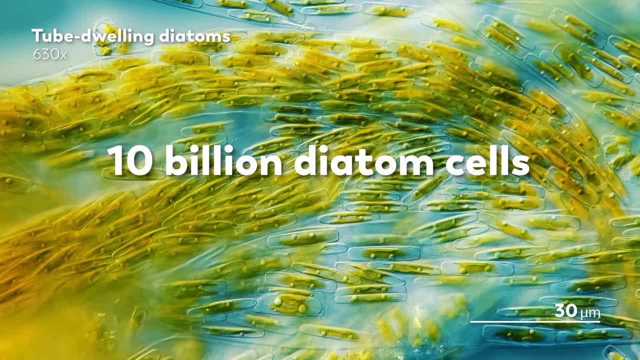 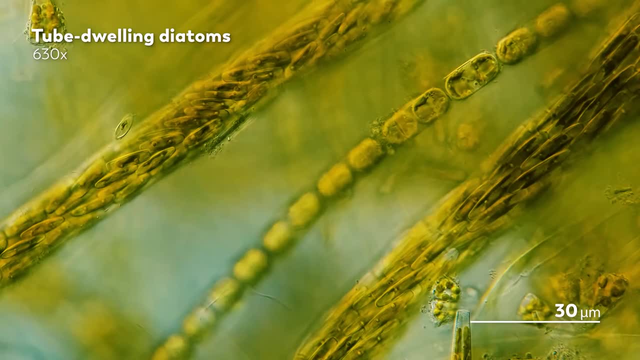 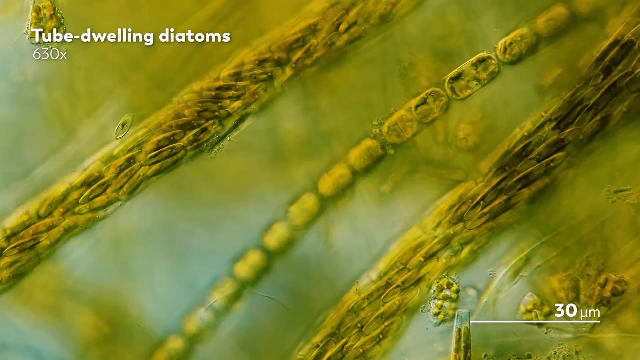 I mean there were more than 10 billion diatom cells living in tubes per square meter. These tubular colonies start with one diatom secreting a thread of mucus from a pore which it weaves into a tube. Living in a mucus tube might not have the same. 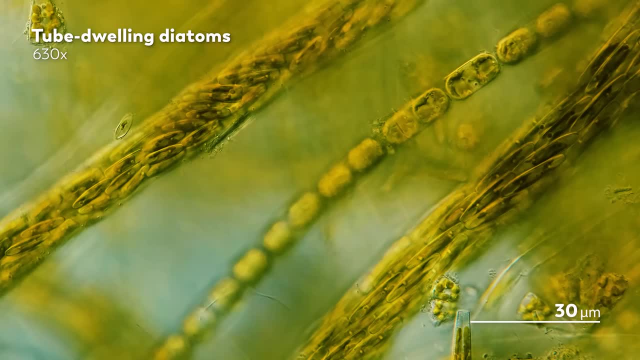 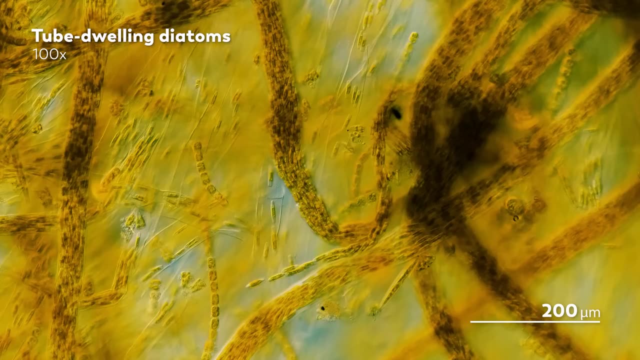 relationship to a diatom, but it's a different type of diatom feel as the diatom stained glass shells. But diatoms don't have much need for romance. As the tube gets longer and longer, the cell reproduces asexually, dividing and populating. 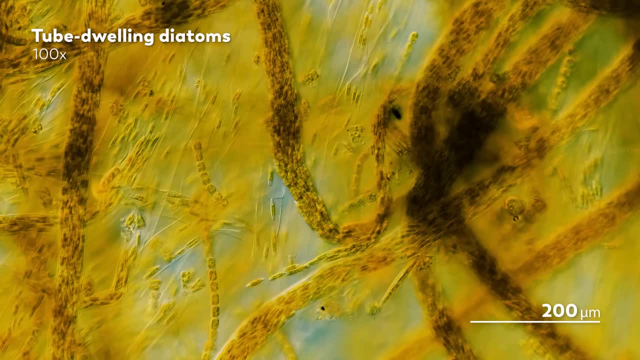 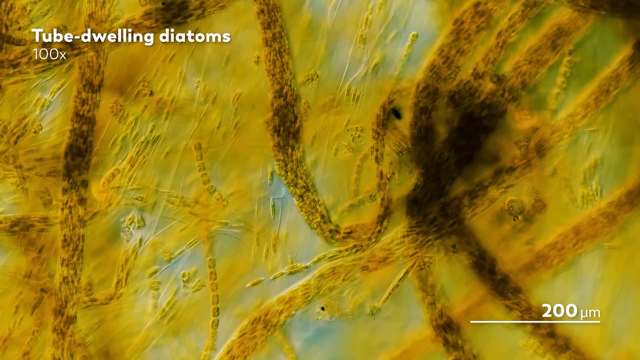 the tube with more cells like it so they can travel through their shared home and add to it. With every cell, a new roommate and construction worker is added, a cell that can be used to build a new home. And when the cell is built, it can be used to build a new home. 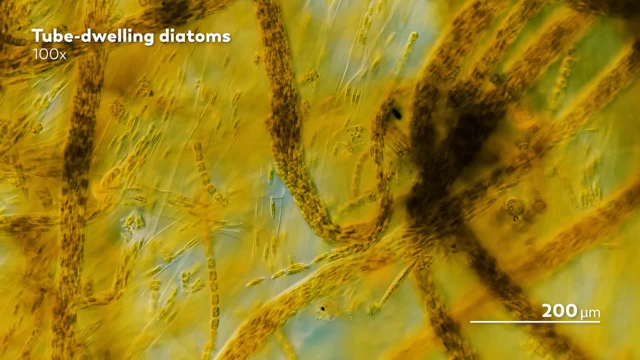 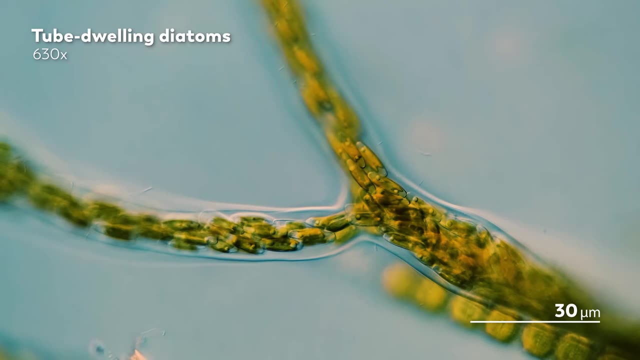 A cell that can strengthen and add to the tube by producing more mucus. At times the cells might reproduce faster than the tube can expand, at which point they might start to create a little side tunnel. Their tube is a colony and they might end up attached to surfaces like sand particles. 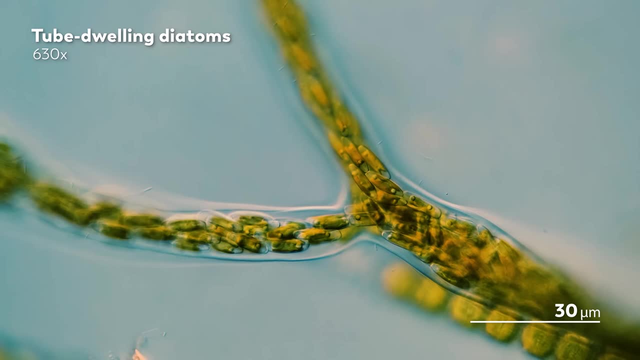 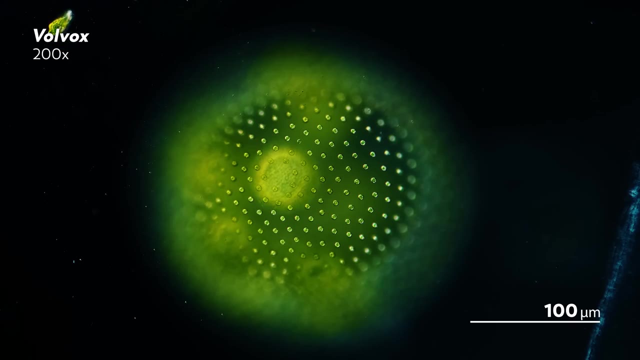 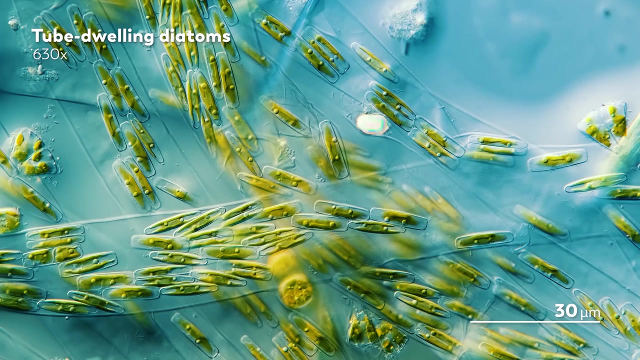 or a submerged Icelandic dock, And they're kind of similar to colonies we've seen on this channel, like volvox and their spherical gatherings. One thing that's strange, though, is that, based on what little we know about these tubes, it doesn't seem as if these diatoms do much to coordinate their activity. 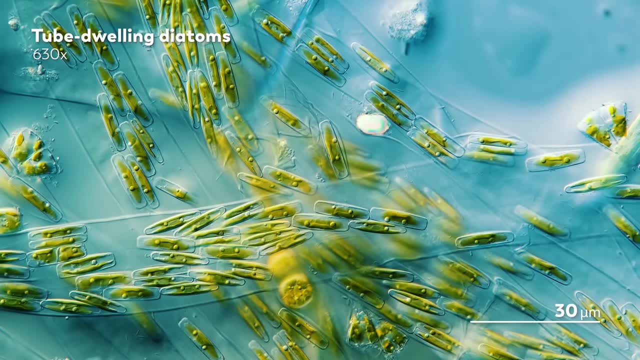 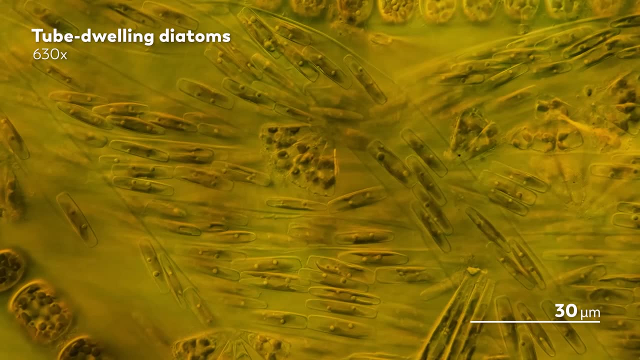 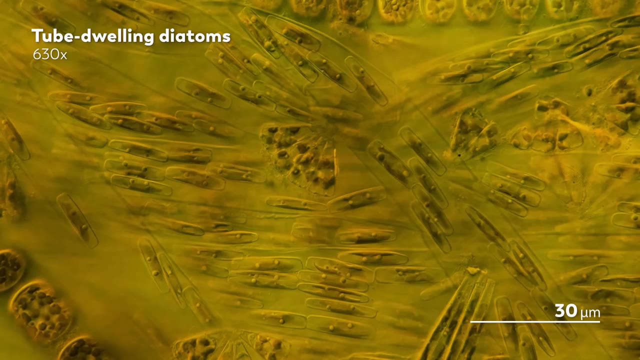 This is different from volvox, where various cells take on different functions and they work together to create a better life for everyone. But some of these diatoms act like they've constructed a crowded city street just to ignore each other. A group of co-workers who don't even 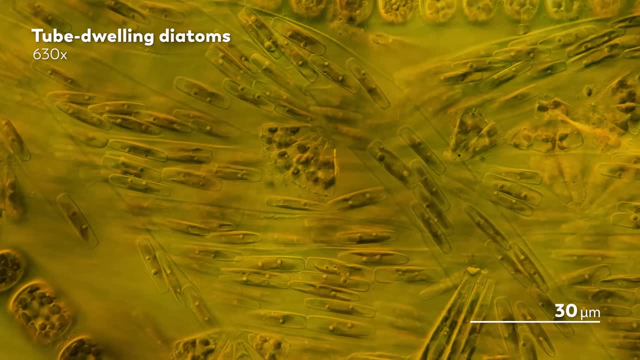 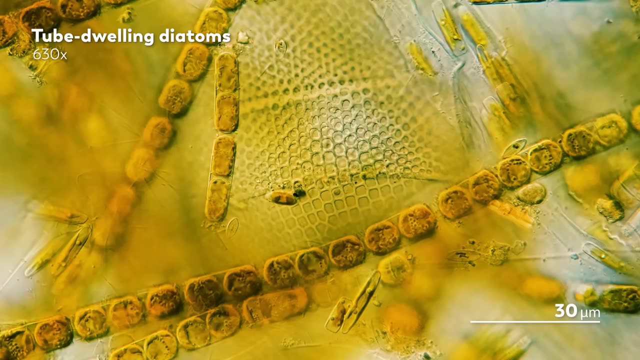 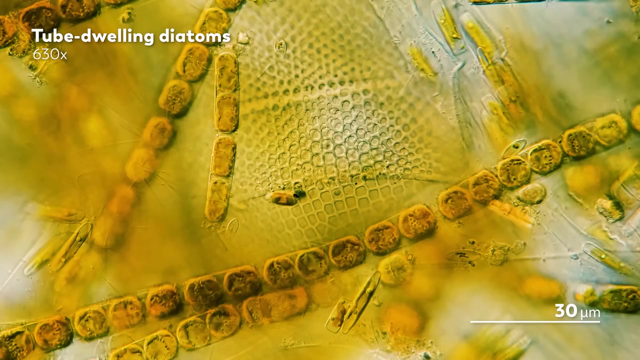 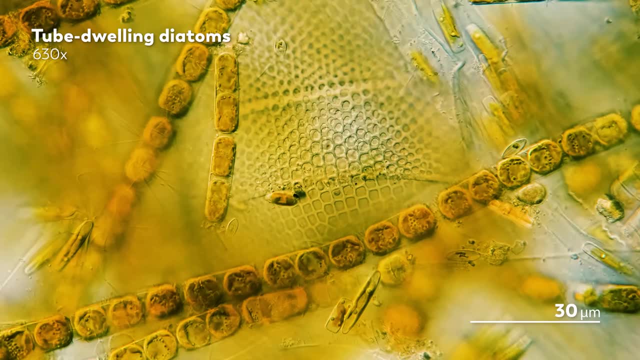 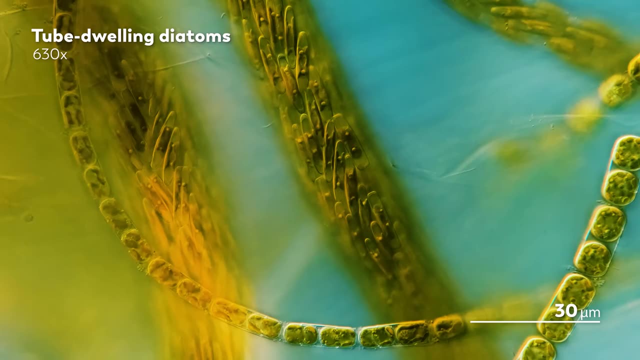 Otherwise, why bother with the time and energy it takes to start making a tube and to keep adding to it? The tube might be a form of protection, making the diatoms too big for microbial predators to consume, But it's probably also a way to help the diatoms. 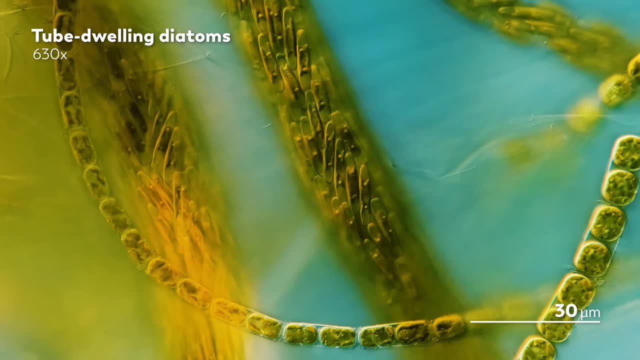 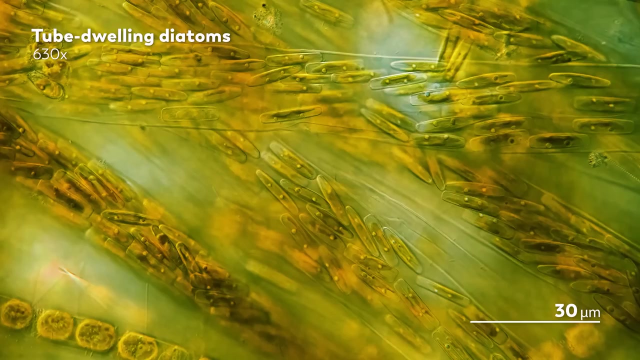 access light through a few different mechanisms. To start, the tubes help lift the diatoms away from the substrate they might have sunk to, raising them towards any light that might penetrate the water. And as they float in the water, the tubes allow the diatoms to move with the rhythm of the waves. 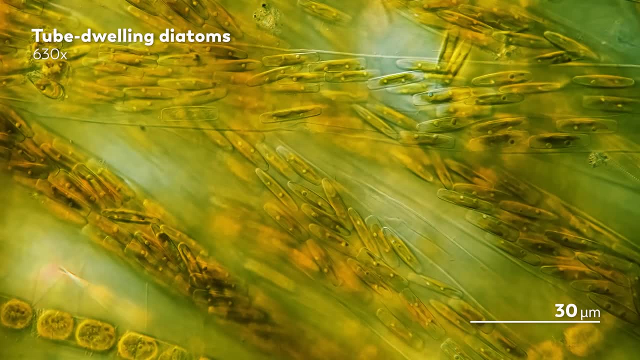 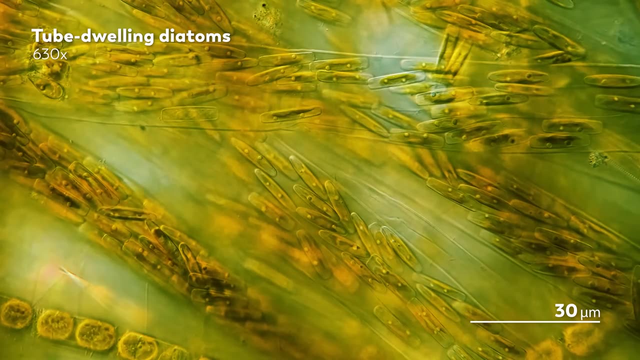 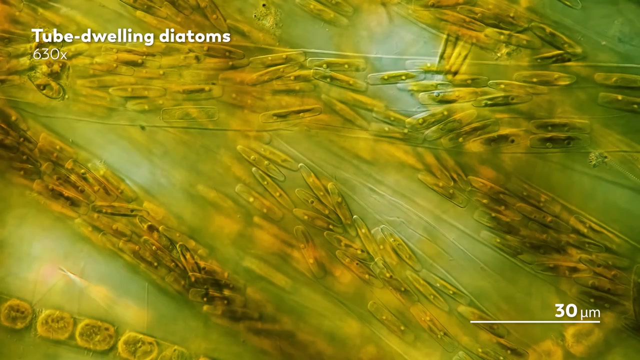 illuminating all sides in the process. At least that's one of the possibilities for why these diatoms turn to tubes. But stepping back from the why, it's like we're starting to see more of who diatoms are. They're builders. They may have never set out to become that, but their approach to the world 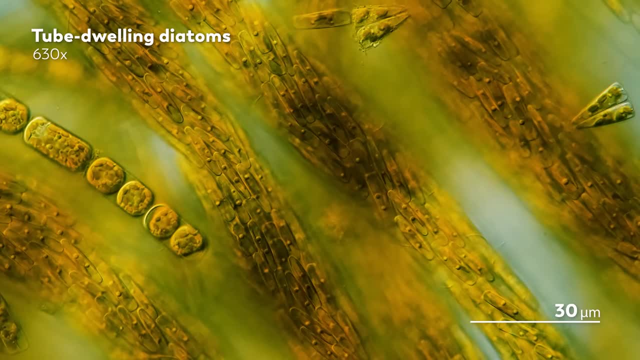 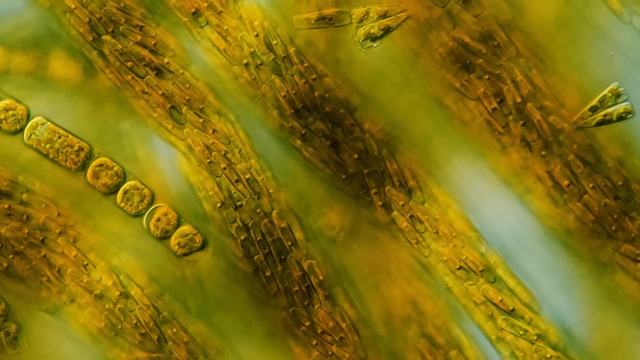 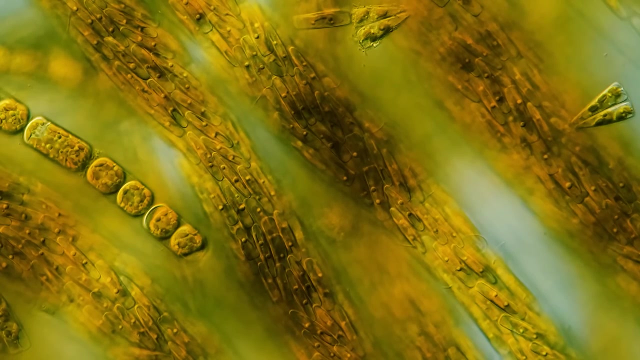 around them has been to build, to assemble, to make something functional and beautiful, even if the beauty is not the point. Thank you for coming on this journey with us as we explore the unseen world that surrounds us, And thank you to Squarespace for sponsoring this episode. 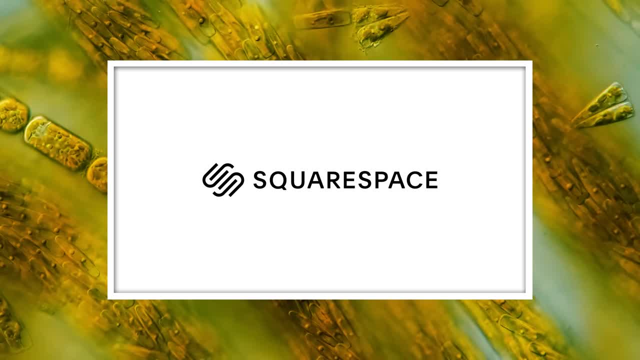 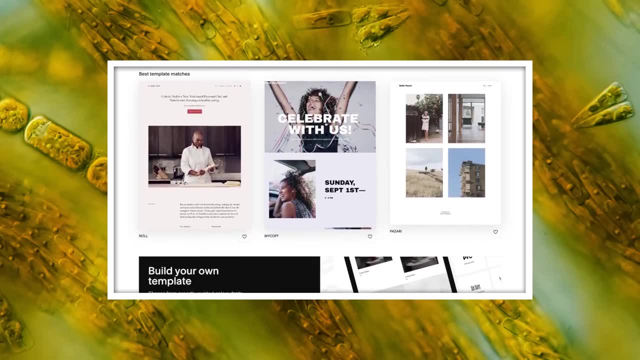 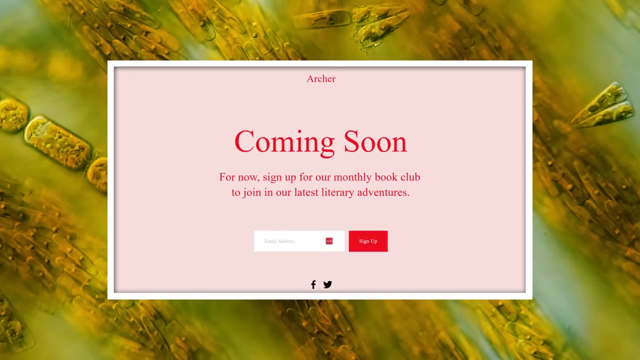 Squarespace gives people a powerful and beautiful online platform from which to create their website. So, whether you're looking to create an online portfolio, start a blog or open an online store, Squarespace can help you out. Maybe it's time for you to take your bookstagram to the next level by 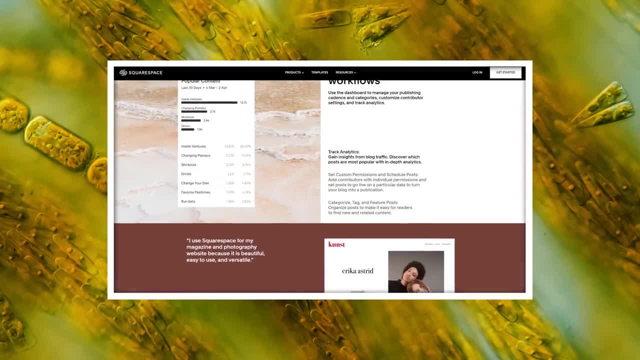 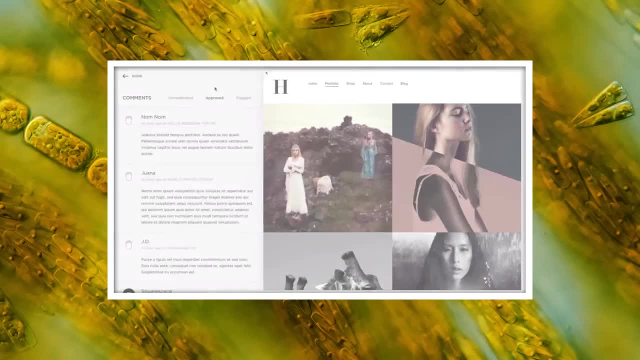 starting a whole book review blog. Well, Squarespace has the tools you need. They make it super simple to categorize, schedule and share your blog posts, And with Squarespace you can interact with your community of fellow book lovers. 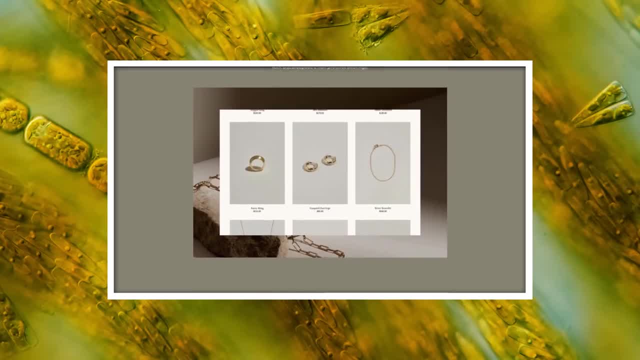 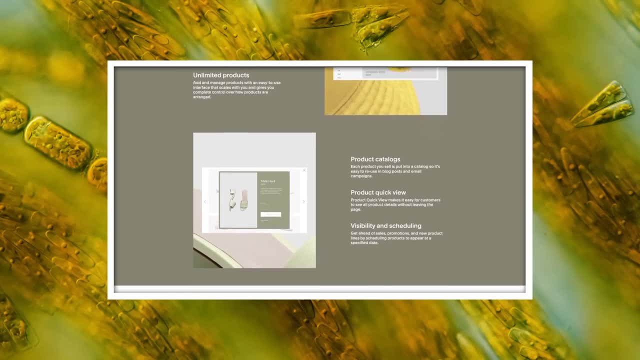 through threaded comments and replies. And if you decide you want to start selling custom bookmarks and book sleeves, Squarespace can help you out there as well. Squarespace is already a powerful e-commerce platform, but you can even go the extra mile and add third-party extensions. 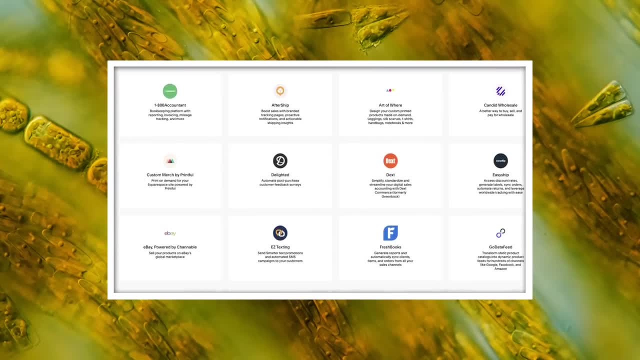 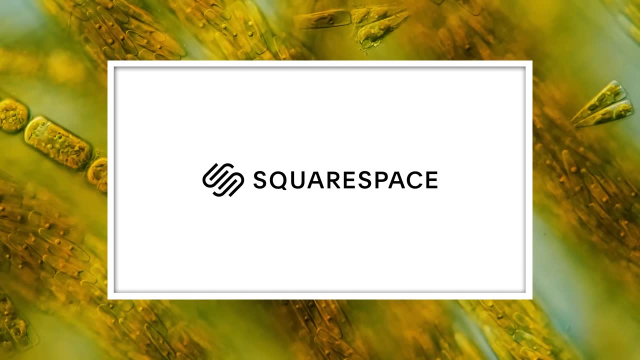 to help you manage inventory, streamline bookkeeping and ship products across the world. And you can do all of this with Squarespace. So go to squarespacecom to sign up for a free trial And when you're ready to launch, go to squarespacecom. slash microcosmos. 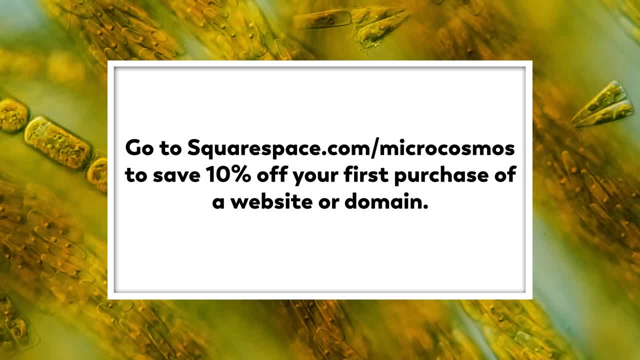 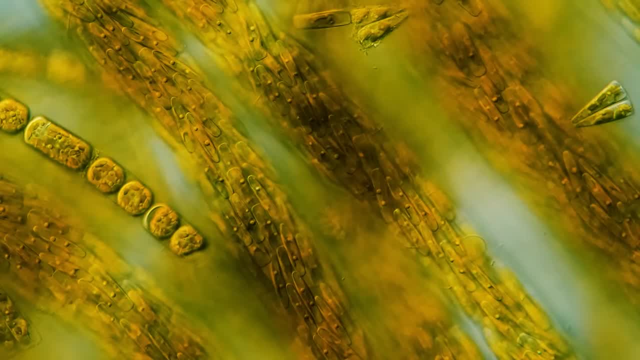 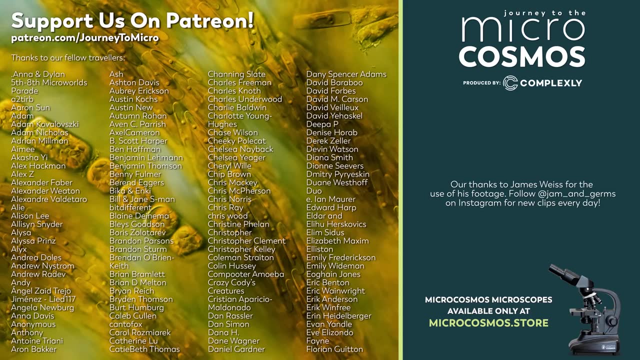 to save 10% off your first purchase of a website or domain. The names on the screen are our Patreon patrons. These are the people who have decided to directly support this channel over at patreoncom slash journeytomicrocosmos, And if you're new to Squarespace, we're here to help. 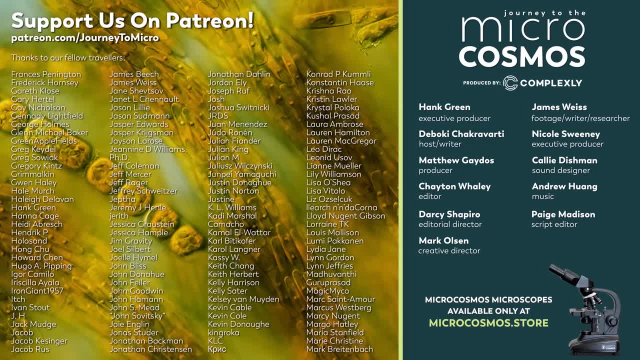 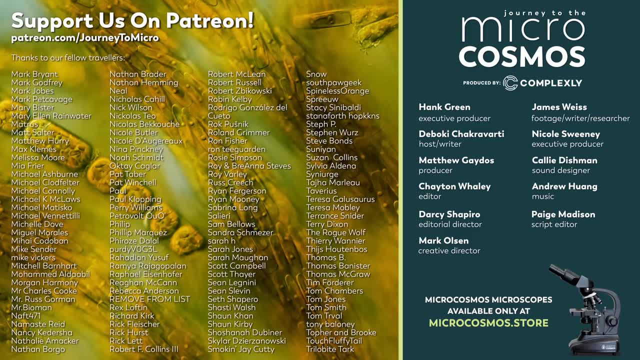 So go to squarespacecom. slash journeytomicro. so we always want to take this time at the end of our videos to thank them for their support. If you want to see more from our master of microscopes, James Weiss, you can check out Jam and Germs on Instagram and TikTok. 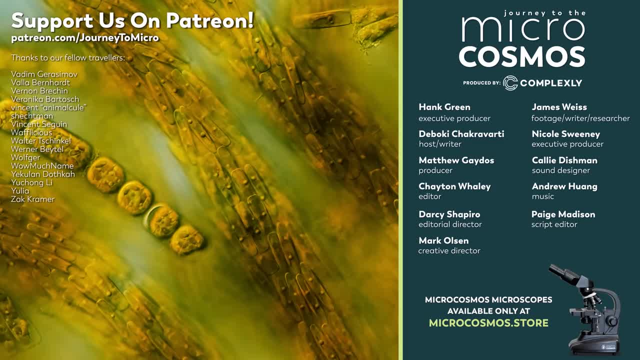 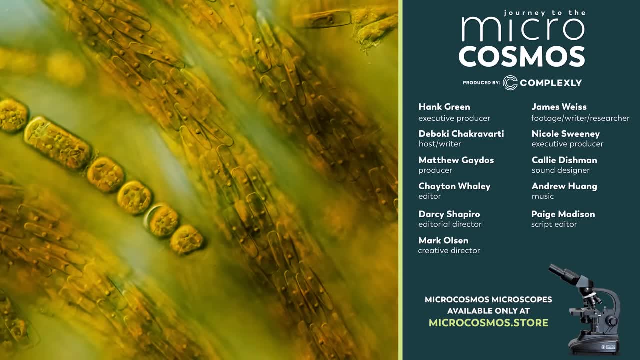 And you can also find Journey to the Microcosmos on TikTok now. if you want some micro microcosmos And if you want to see more from us here on YouTube, there's always a subscribe button somewhere nearby, And we'll see you next time on Journey to the Microcosmos. Have a great day. 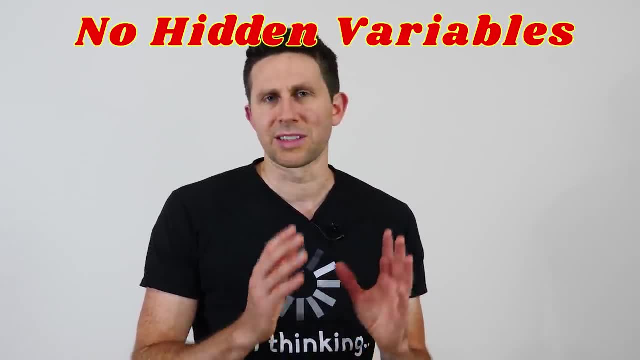 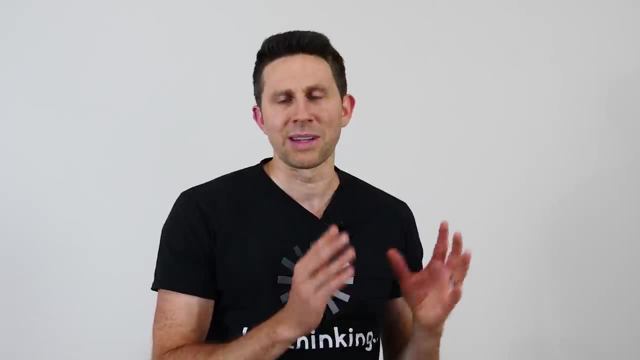 Hey everyone. today I'm going to be showing you how there can be no hidden variables in quantum mechanics. And to start off, let me show you what a hidden variable is, and then I'll explain why they can't happen in quantum mechanics. I have a tube here with some strings. 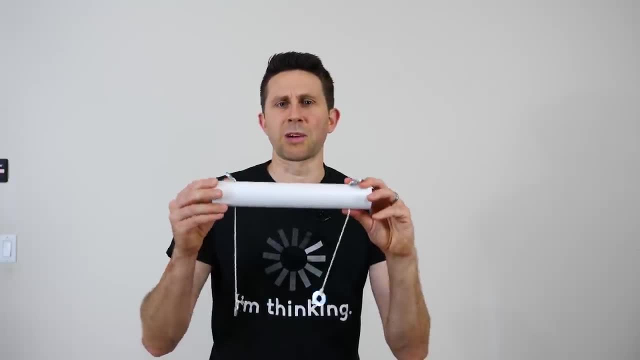 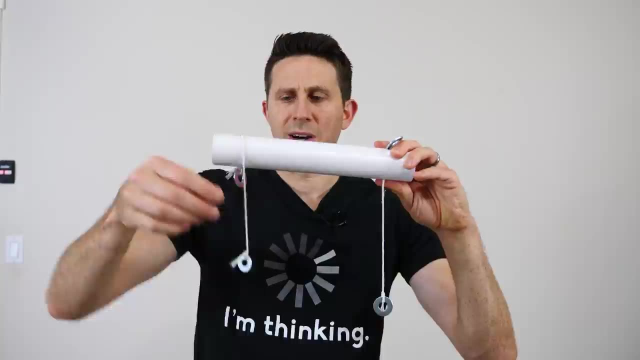 through it. I want you to make some predictions on what you think will happen when I pull certain strings, based on what you observe here. So first I'm going to pull up the top string- You can see that it pulls up the bottom string as well- And then, on the other side,